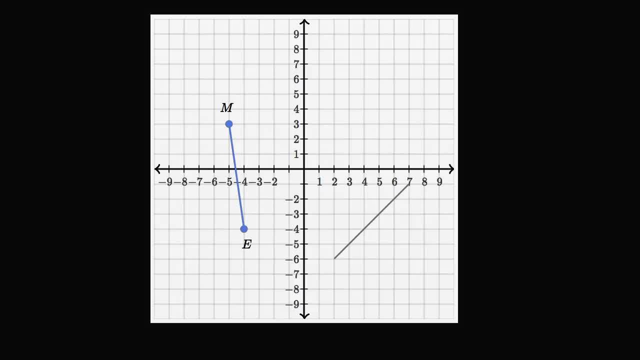 So let me get my scratch pad out and I copied and pasted the same diagram And the line of reflection, one way to think about it. we want to map point E to this point right over here. We want to map point M to this point over here. 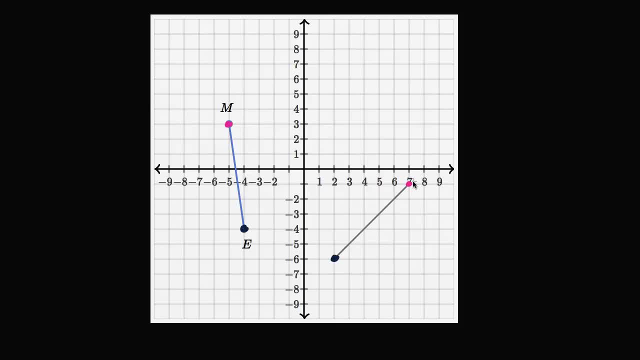 And so, between any point and its corresponding point on the image after the reflection, these should be equidistant. This and this should be equidistant from the line of reflection. This and this should be E and this point should be equidistant from the line of reflection. 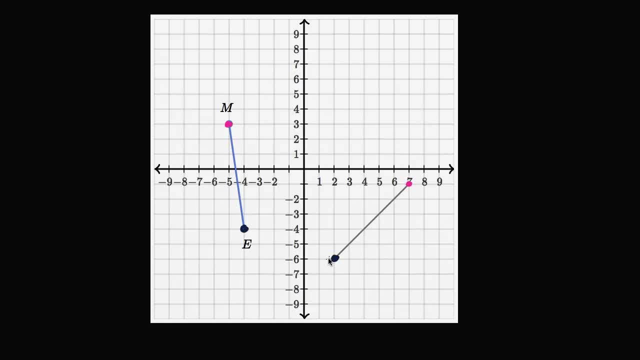 Or another way of thinking about it. that line of reflection should contain the midpoint between these two magenta points and it should contain the midpoint between these two deep navy blue points. So let's just calculate the midpoints. So we could do that with a little bit of mathematics. 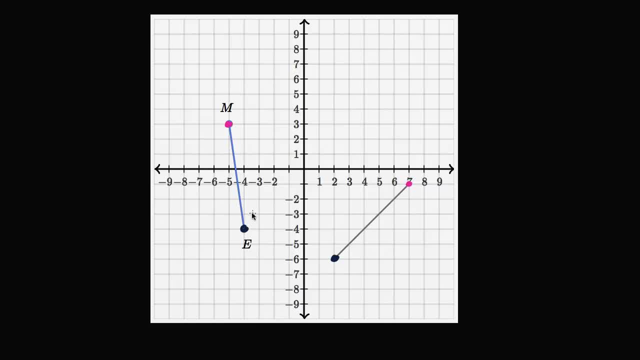 The coordinates for E right over here, that is. let's see that is: x equals negative four, y is equal to negative four And the coordinates for the corresponding point to E in the image. this is: x is equal to two, x is equal to two and y is equal to negative six. 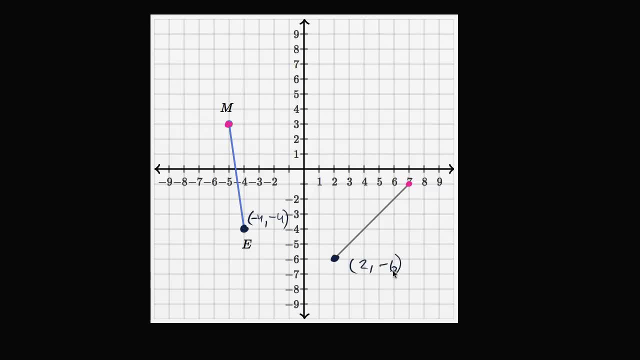 So what's the midpoint between negative four, negative four and two comma negative six? Well, you just have to take the average of the x's and take the average of the y's. Let me do that. I'll actually do it over here. 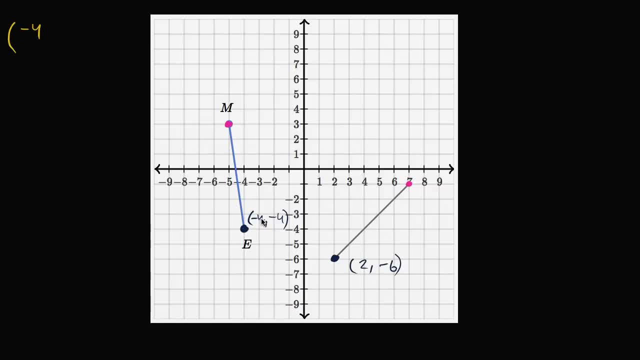 So if I take the average of the x's, it's going to be negative four negative four plus two plus two over two. That's the average of the x's. And then the average of the y's is going to be negative four plus negative six over two. 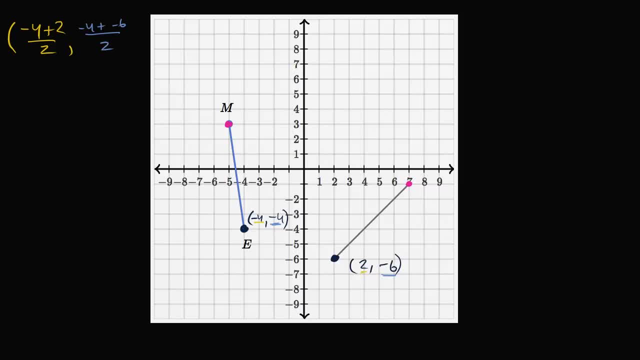 Negative four plus negative six over two. And then close the parentheses, Let's see: negative four plus two is negative two divided by two is negative one, So it's going to be negative one comma. negative four plus negative six is the same thing as negative four minus six. 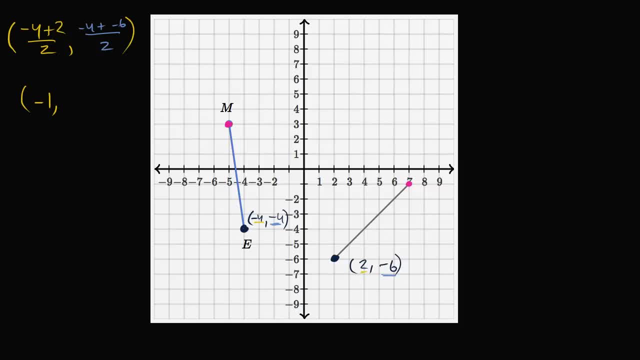 which is going to be negative. ten divided by two is negative five- Let me do that in a blue color, so you see where it came from- is going to be negative five. So there you have it. That's going to be the midpoint between E and the corresponding point on its image. 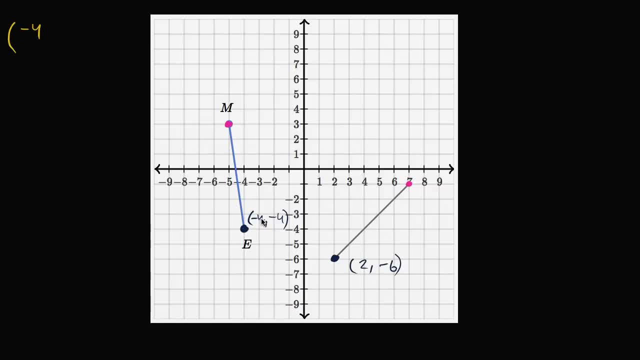 So if I take the average of the x's, it's going to be negative four negative four plus two plus two over two. That's the average of the x's. And then the average of the y's is going to be negative four plus negative six over two. 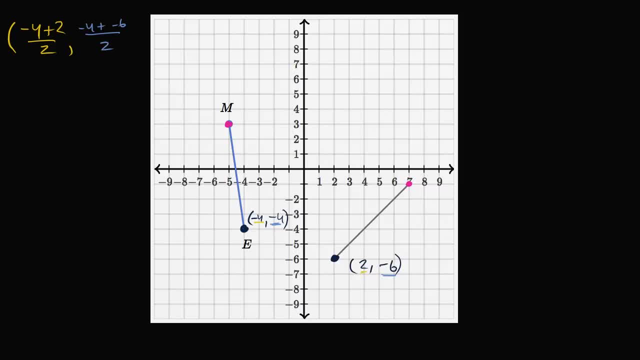 Negative four plus negative six over two. And then close the parentheses, Let's see: negative four plus two is negative two divided by two is negative one, So it's going to be negative one comma. negative four plus negative six is the same thing as negative four minus six. 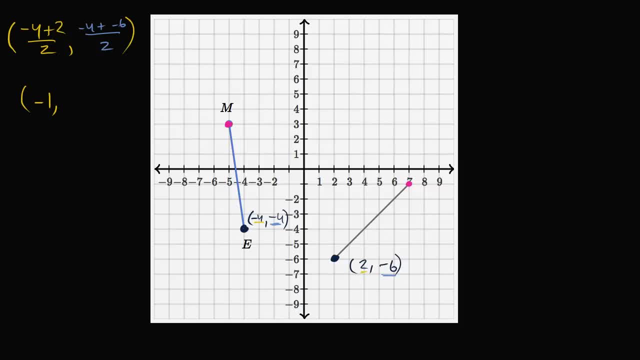 which is going to be negative. ten divided by two is negative five- Let me do that in a blue color, so you see where it came from- is going to be negative five. So there you have it. That's going to be the midpoint between E and the corresponding point on its image. 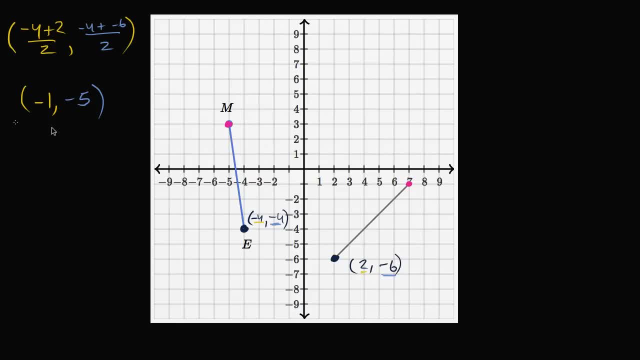 So let's see if I can plot that. So this is going to be: this point right over here is going to be: negative one comma, negative five. So x is negative one, y is negative five. So it's this point right over here. 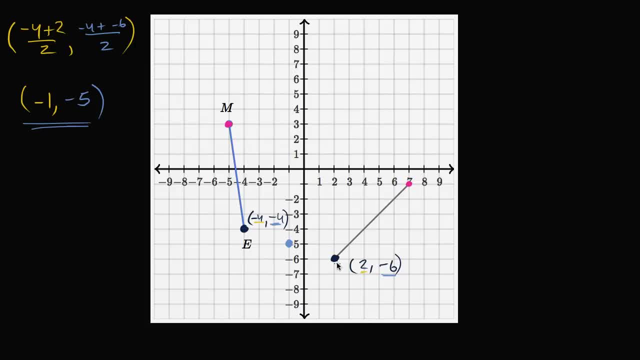 And it does indeed look like the midpoint. It looks like it's equidistant between E and this point right over here, And so this should sit on the line of reflection. So now let's find the midpoint between M and this point right over here. 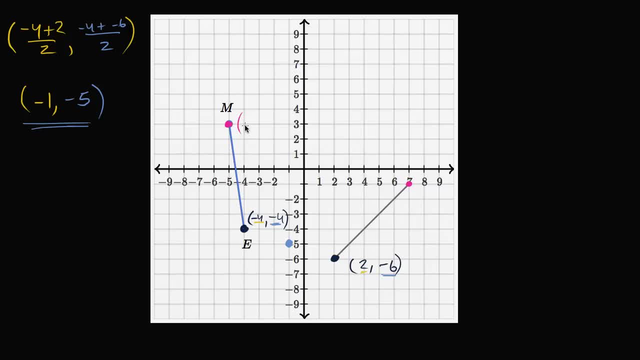 The coordinates of M are: x is negative five and y is equal to three. The coordinates here are: x is equal to seven and y is equal to three And y is equal to negative one. So the x-coordinate of the midpoint is going to be the average of the x's here. 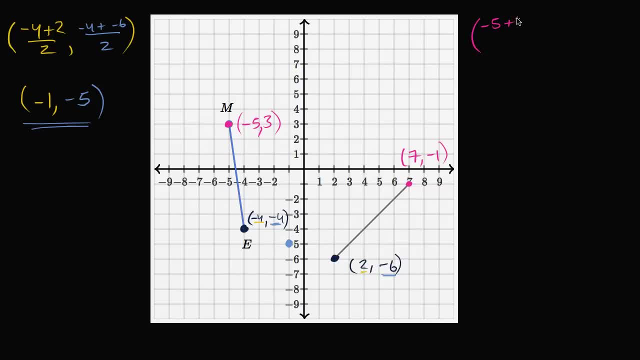 So let's see It's going to be negative. five plus seven over two, and the y-coordinate of the midpoint is going to be the average of the y-coordinates. So three plus negative, one over two, Let's see negative. five plus seven is positive. two over two is one. 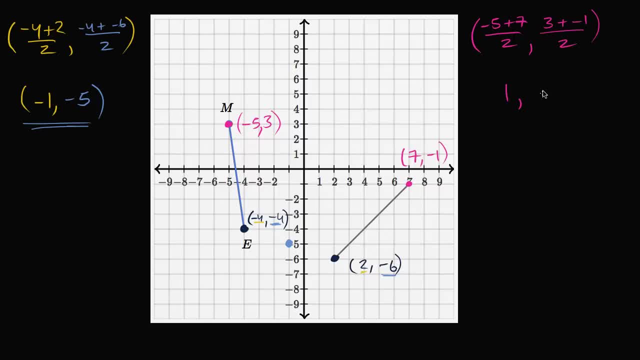 Three minus one, three plus negative one. that's positive, two positive. two over two is one. So the point one comma one is the midpoint between these two. so one comma one, just like that. So the line of reflection is going to contain: 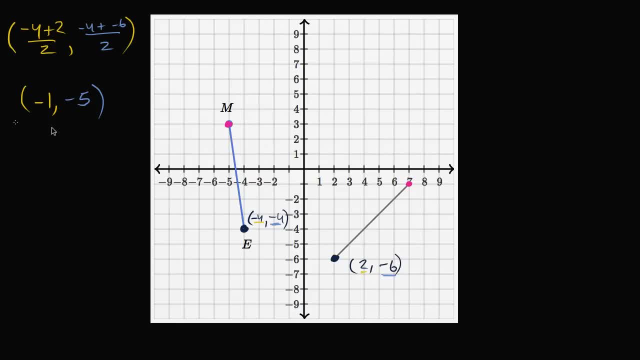 So let's see if I can plot that. So this is going to be: this point right over here is going to be: negative one comma, negative five. So x is negative one, y is negative five. So it's this point right over here. 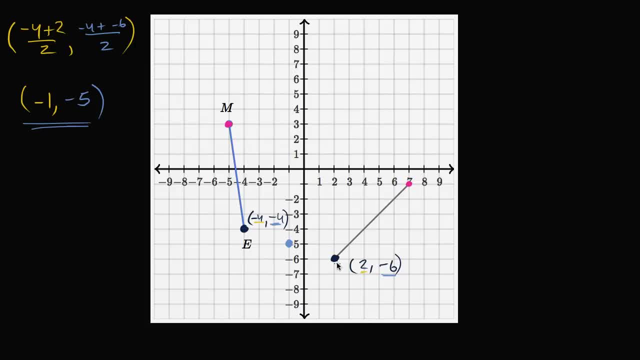 And it does indeed look like the midpoint. It looks like it's equidistant between E and this point right over here, And so this should sit on the line of reflection. So now let's find the midpoint between M and this point right over here. 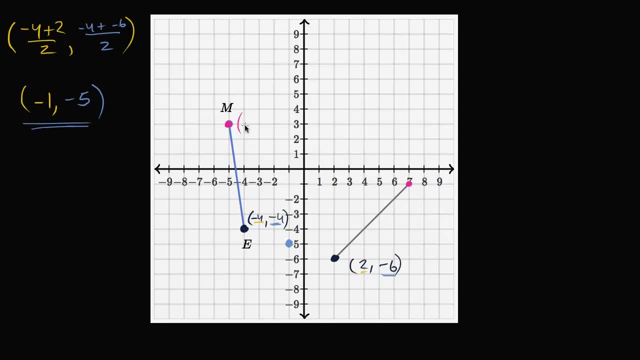 The coordinates of M are: x is negative five and y is equal to three. The coordinates here are: x is equal to seven and y is equal to three And y is equal to negative one. So the midpoint, the x coordinate of the midpoint. 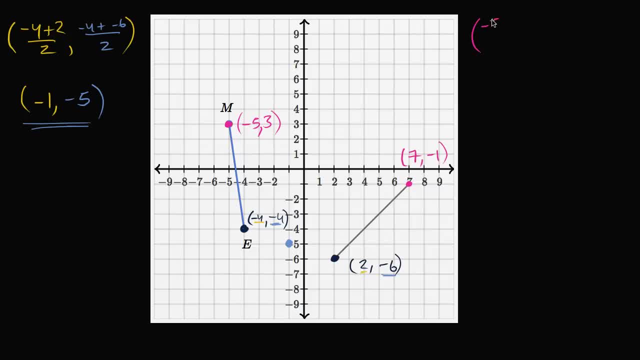 is going to be the average of the x's here. So let's see it's going to be negative five plus seven over two And the y coordinate of the midpoint is going to be the average of the y coordinates. So three plus negative one over two. 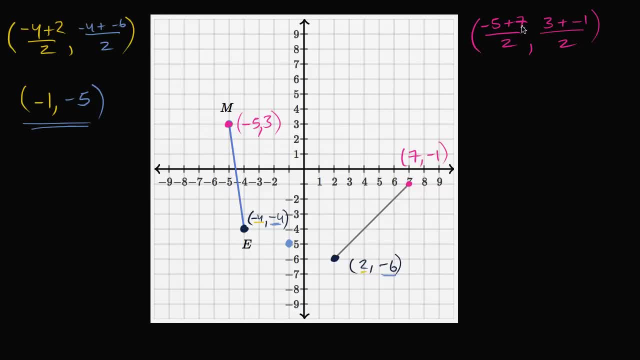 Let's see: negative: five plus seven is positive. two over two is one. Three minus one. three plus negative one. positive. two over two is one. So the point one comma one is the midpoint between these two. so one comma one, just like that. 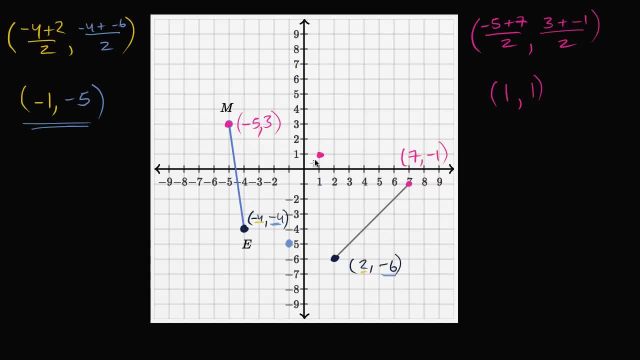 So the line of reflection is going to contain these two points, and two points define a line. In fact, I could let me draw the line of reflection, just because we did all of this work. The line of reflection is going to look something like: 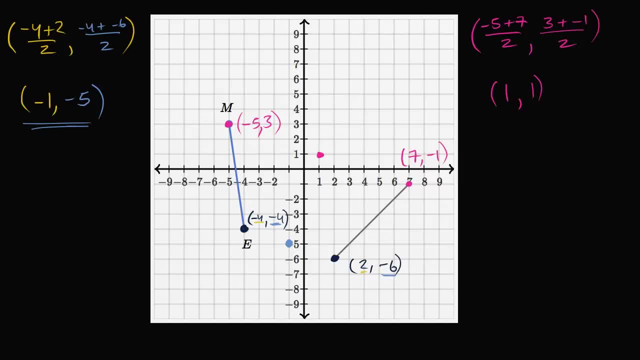 these two points, and two points define a line. In fact, I could let me draw the line of reflection, just because we did all of this work. The line of reflection is going to look something like: is going to look something like: 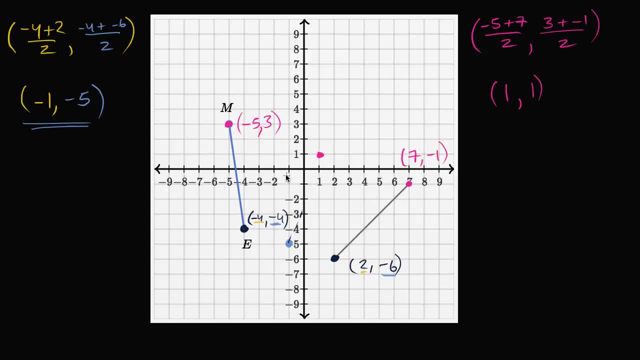 is going to look something like: oh, I need- I want to draw this a little bit straighter than that- It's going to look something like. it's going to look something like something like this, And this makes sense, that this is a line of reflection. 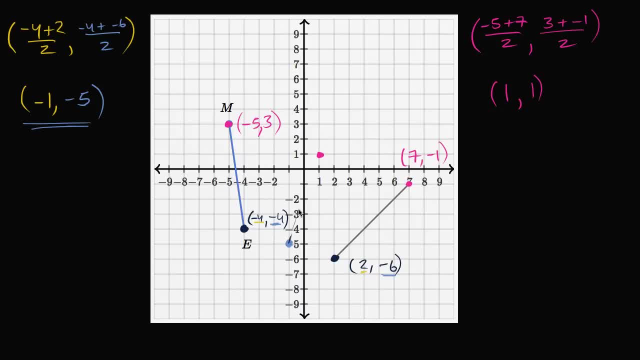 I missed that magenta point a little bit, So let me go through the magenta point. Okay, there you go. This makes sense that this is a line of reflection, because you see that every you pick an arbitrary point on segment ME, say that point. 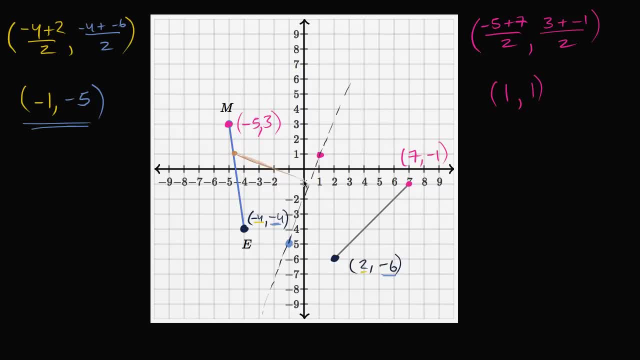 and if you reflect it over this line, it's this: this is its shortest distance from the line. You just go onto the other side of the line, an equal distance, and you get to its corresponding point on the image. So it makes a lot of sense that these are mirror images. 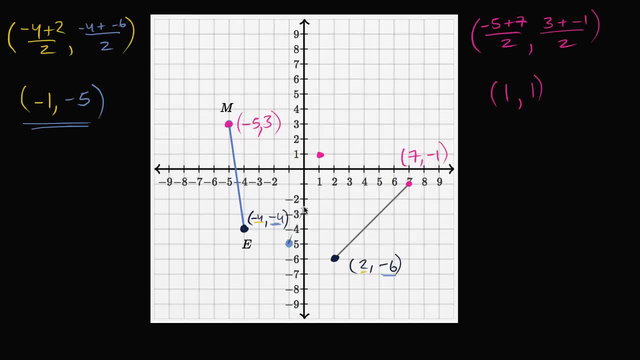 oh, I need to. I want to draw this a little bit straighter than that. It's gonna look something like. it's gonna look something like something like this, And this makes sense that this is a line of reflection. I missed that magenta point a little bit. 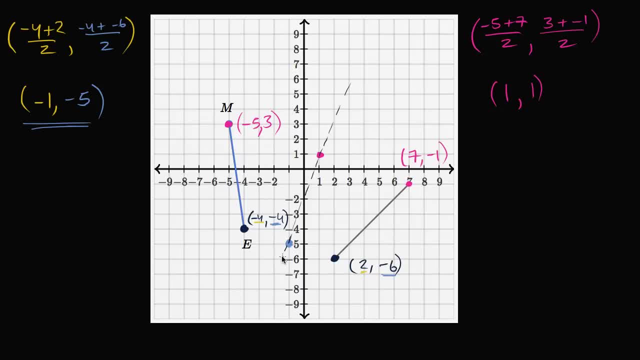 So let me go through the magenta point. Okay, there you go. This makes sense that this is a line of reflection, because you see that every you pick an arbitrary point on segment ME, say that point and if you reflect it over this line, 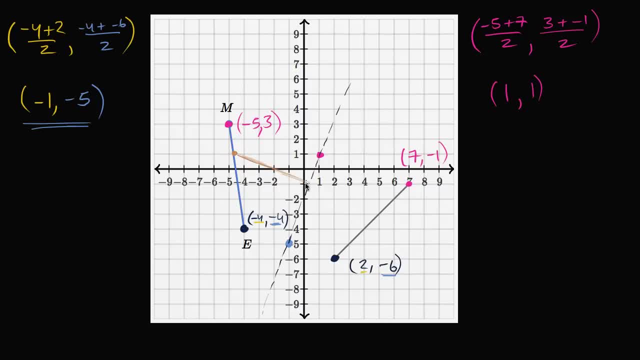 it's this: this is its shortest distance from the line. You just go onto the other side of the line, an equal distance, and you get to its corresponding point on the image. So it makes a lot of sense that these are mirror images, if this is kind of the mirror here.